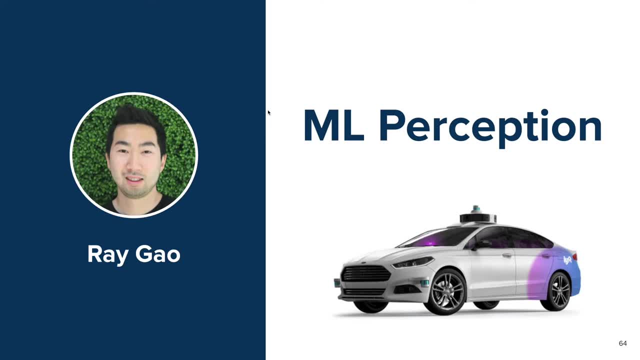 Hello, my name is Ray and today I'm going to talk to you about the latest trends and state of machine learning in perception. This is the earliest part of the autonomy stack that uses raw sensor inputs to understand the driving environment around us. So what are we going? 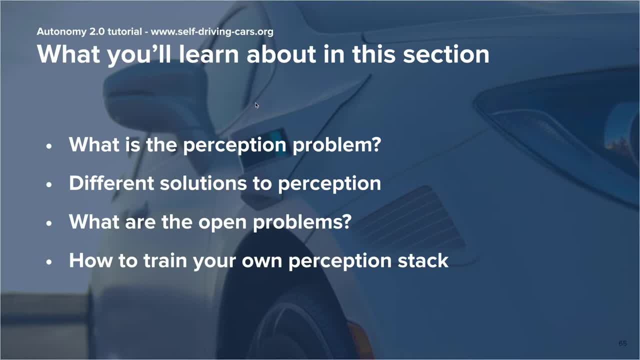 to learn in this section. First we'll talk about what is the perception problem. Next we'll talk about different solutions to perception, Then what are the open problems in perception And then finally, how to train your own perception stack with the L5 kit. 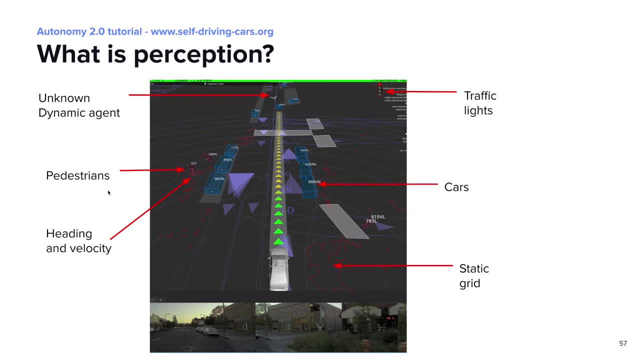 So what is perception At a high level? perception is about creating an encoding of the driving environment that can then be used for downstream tasks such as motion prediction and planning. This is an example of our perception system. You can see a scenario where the self-driving 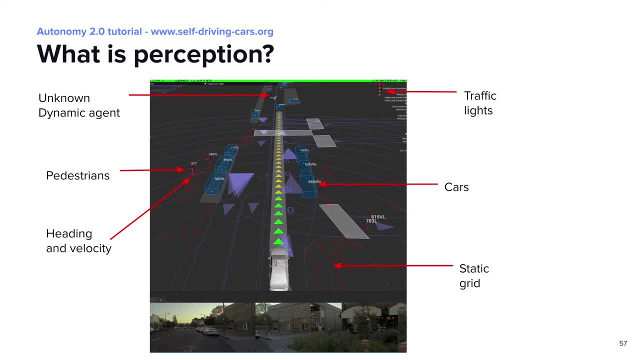 car is just driving down the road and the car is driving down the road, And then you can see the car driving down a road. There are cars on the side of the road represented by the blue bounding boxes. From the left you'll see some pedestrians shown by purple. 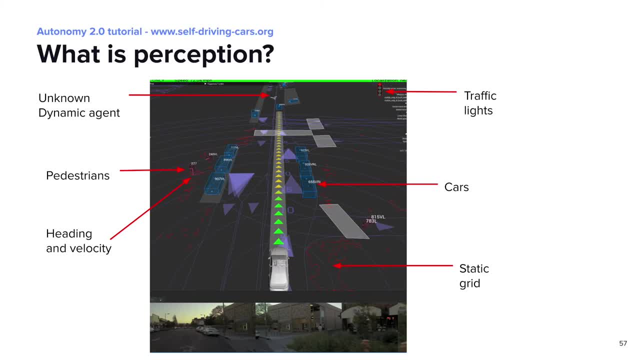 bounding boxes. They have lines coming out of them showing which direction they're headed and how fast they're going. There's a traffic light indicator at the top right showing us the state of the traffic light ahead. There are some gray boxes in the distance telling. 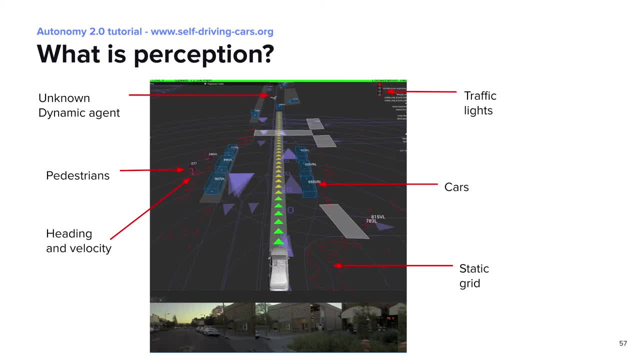 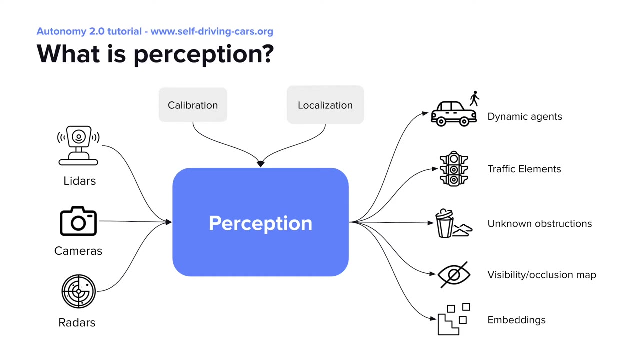 us they're moving objects, but we don't know what they are. And finally, there are some red outlines. These are polygons that show us static objects such as bushes and buildings. To generate these type of outputs, we need a perception stack. This is usually some collection. 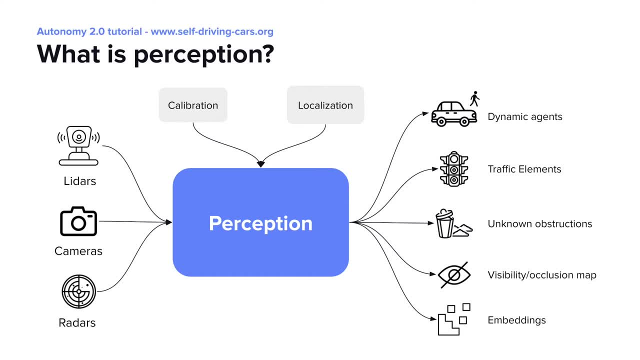 of algorithms that take in a set of sensors and other information to produce the type of outputs we were describing. Some examples include lidars, cameras and radars as sensors. Lidars use laser beams to provide accurate depth information. Cameras mimic the vision. 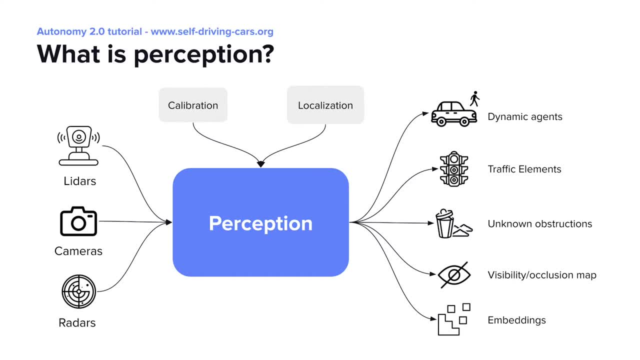 system of a human eye, Radars tend to provide the most accurate velocity information of moving objects. These are no where near all the possible inputs, but these are the most common ones. We typically also need calibration and localization. to ask about the location of the sensors with 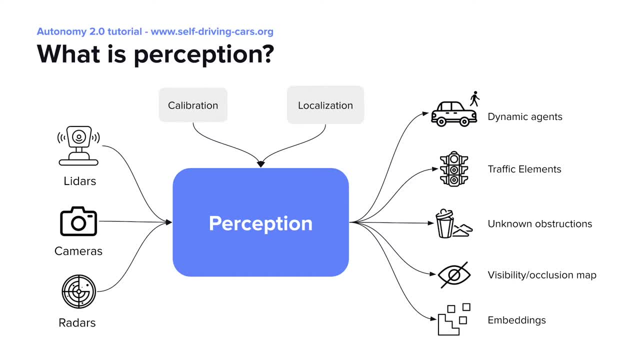 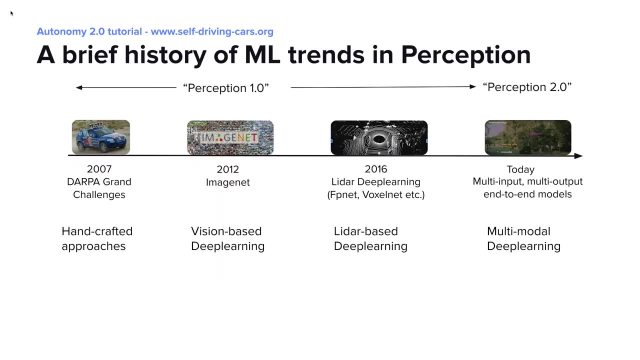 respect to each other and the location of the self-driving car in the world. Some of the first modern perception systems for self-driving cars was conceived around 2007 in the dharka Challenges. They were primarily geometric computer systems that used the Doppler scale to simulate a 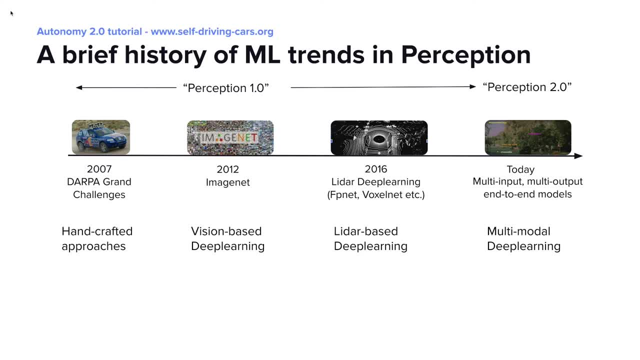 vision-based methods based on handcrafted approaches. In 2012,, after the conception of ImageNet, we started seeing a lot more image-based deep learning methods replace geometric computer vision methods. A few years later, when other sensors became more commonplace, the image-based machine learning methods. 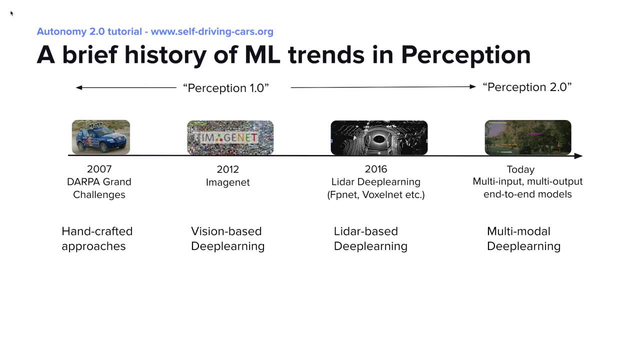 transited over to other spaces, such as LiDAR and radar point clouds. Up to around that point. I would call this state perception 1.0, where perception was a large collection of geometry and machine learning-based methods and there were assembled into a complete perception stack with a huge amount of 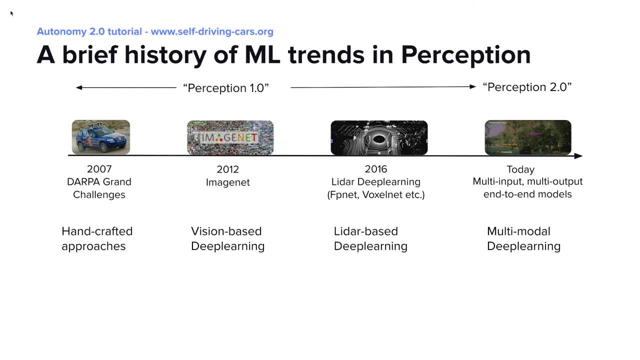 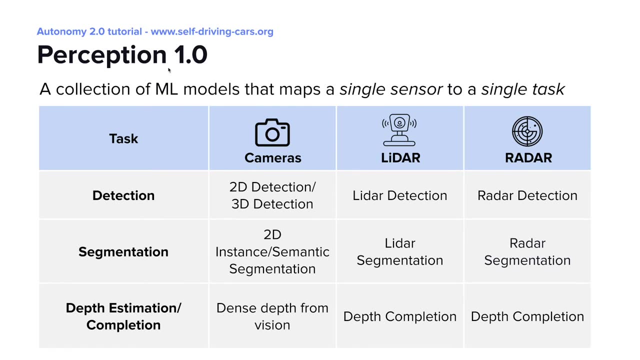 glue code. Today, we're seeing perception becoming much more end-to-end, with fewer models, handling more inputs and producing more outputs. This is what I will call perception 2.0 and where we're headed. Let's dig a bit deeper into what we call perception 1.0.. As previously mentioned, 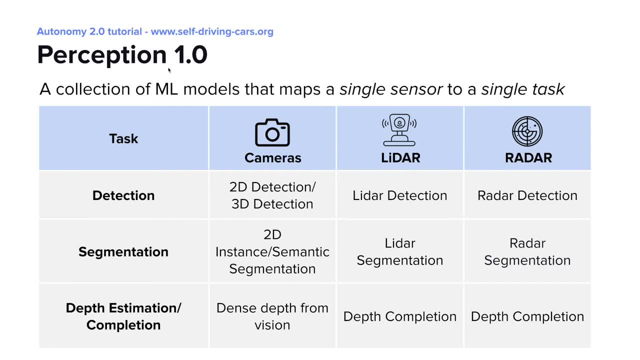 there are typically many types of sensors and we can map them to many tasks. For example, we can perform tasks such as detection, segmentation and depth estimation with either cameras, LiDAR or radar. A typical perception system will then fuse together outputs from these tasks in some pipeline. Note this table. 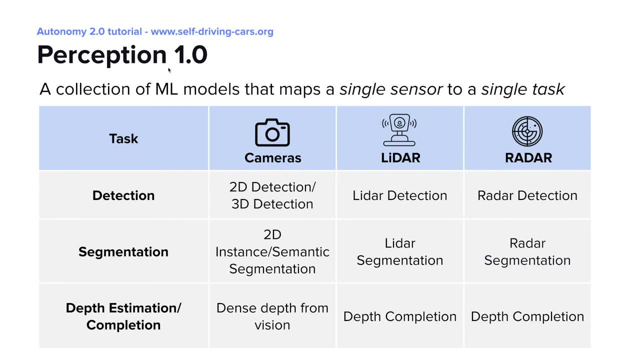 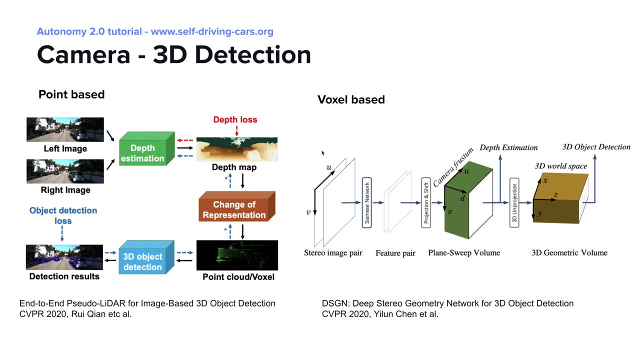 is really just an example of the types of tasks that exist In reality. there are many more types of sensors and tasks. We'll just go over a few examples in this tutorial today. 3D detection with cameras is one of the most common and important tasks in 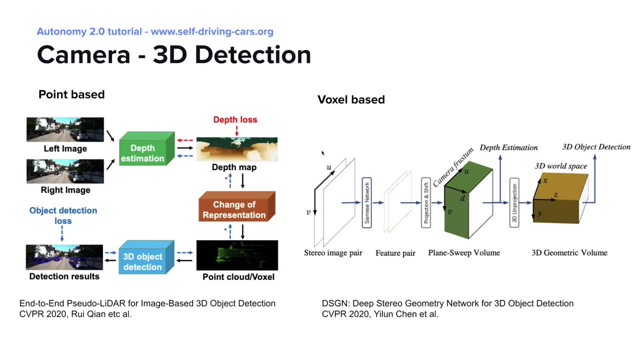 perception. There are typical approaches that operate in point space or voxel space. On the left is a method called pseudo-LiDAR that has recently produced state-of-the-art results in camera-based detection. This approach first generates a dense, depth map from images and then uses 3D LiDAR detection methods to 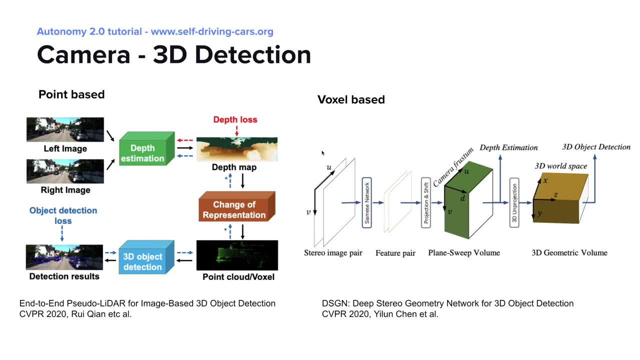 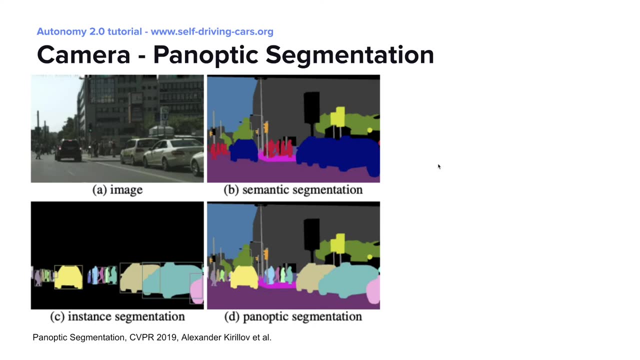 localize objects. Another type is to generate voxel-based feature maps from cameras directly and then use geometry-based detection methods to localize objects. Another type is to generate voxel-based feature maps from cameras directly and then use geometry-based detection methods to localize objects. Another type is to generate voxel-based detection methods to localize objects. Another type of task is panoptic segmentation. This 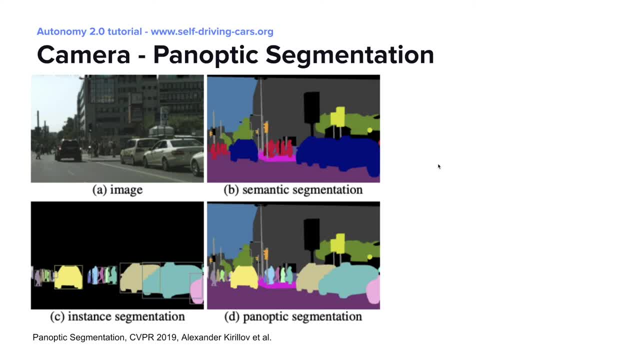 task produces a per-pixel classification for each type of object and for every instance of an object. fusing semantic and instance segmentation: Standard methods for semantic segmentation, such as DeepLab, and instance segmentation, such as MaskR-CNN, can be fused together to produce. 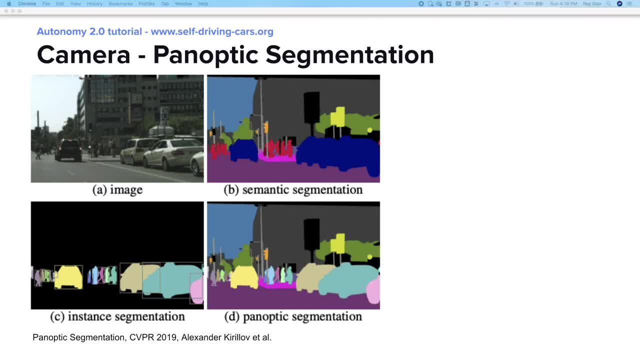 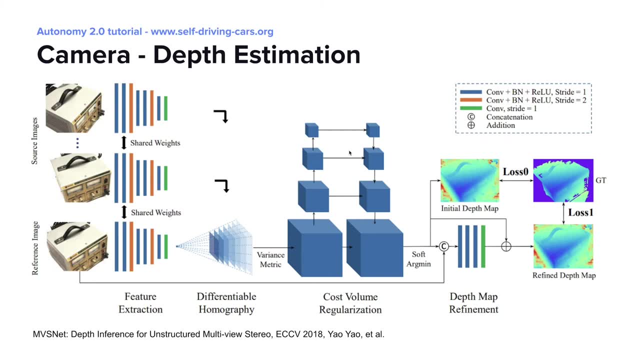 state-of-the-art panoptic segmentation results. Camera depth estimation is another important problem in perception. There exists many such methods for different configurations of cameras, such as Mono, Stereo and MultiView. This example shown here removes the constraint of the structured camera geometries. The MVsSNet uses the idea of a differentiable. 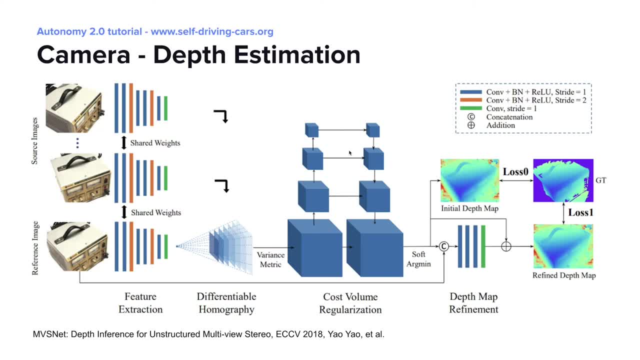 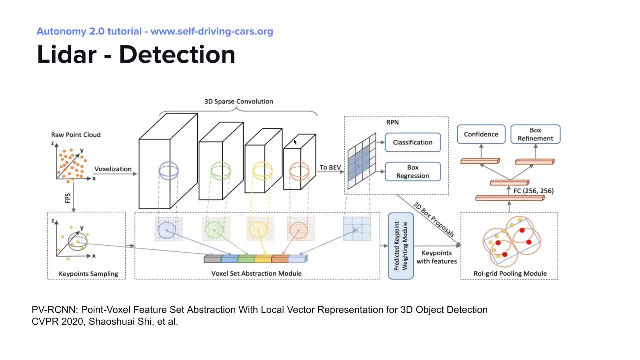 homographic warping layer to produce a 3D cost volume, which then can be used to refine a dense depth map Mirroring 3D detection of cameras. We can do the same with lighter point clouds. The state-of-the-art methods here tend to combine point space and voxel spatial. 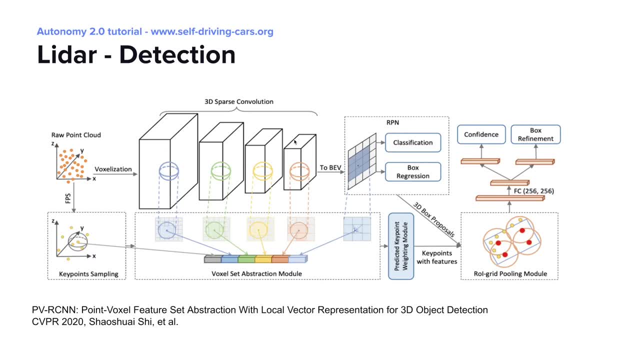 representation. again, Voxel-based methods involve aggregating point information into fixed grids and then applying 2D or 3D convolutions in image-based deep learning methods. This tends to lose fine-grained information, such as locality of points that can easily be retained in point-based methods. however, 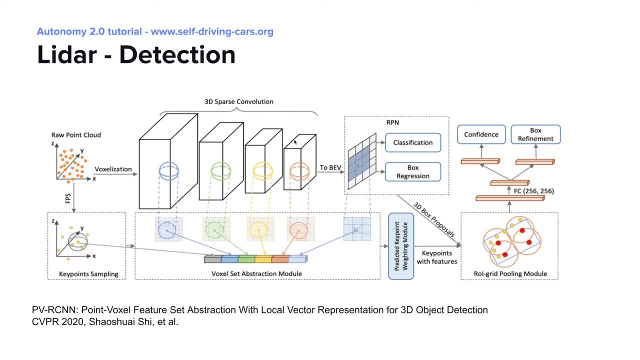 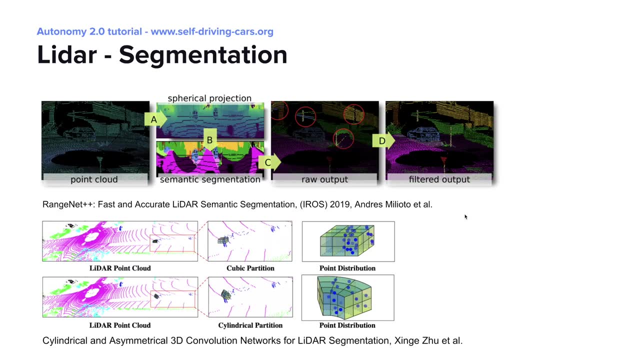 Point voxel fusion methods, where the point features are dependent to voxel features, give the best results. today, LiDAR segmentation is typically done by either converting point clouds to range images and then applying 2D semantic segmentation methods or partitioning points in Cartesian or 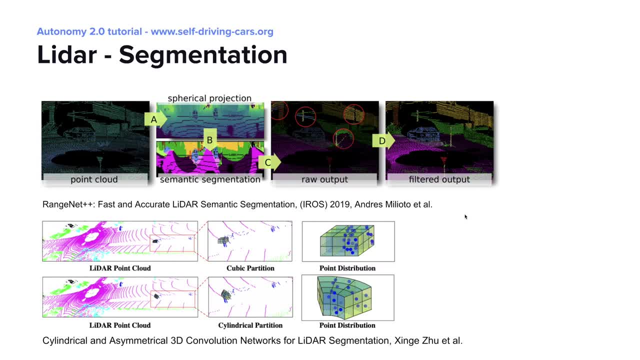 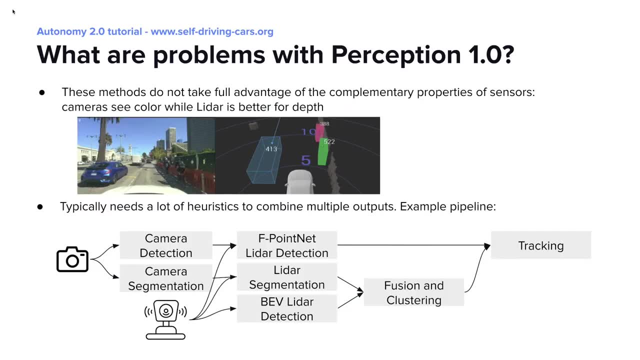 polar coordinate systems and then applying convolutions to produce per-point classifications. What are the problems with perception 1.0?? One issue is that models based on single modalities don't take full advantage of the complementary properties of sensors. For example, LiDAR has excellent depth. 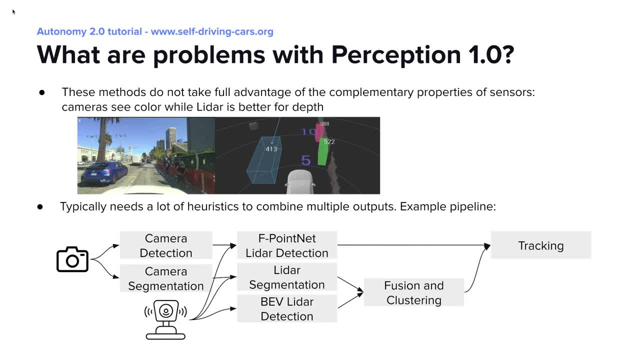 information but can't see color, while cameras are the opposite. In this example scene, a pedestrian and a cyclist are moving very close to traffic and edges of a wall. It will be very difficult in LiDAR space to separate the precise points that. 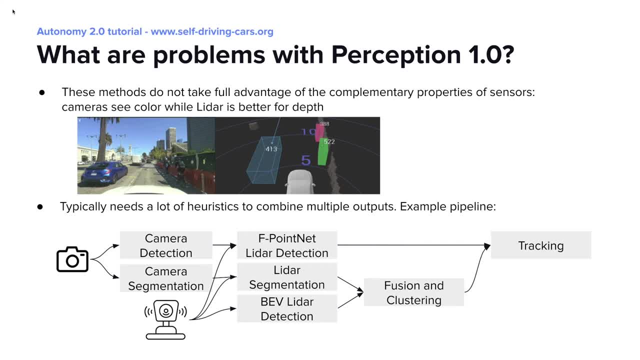 belong to the humans versus the walls. However, from the camera point of view, it should be very easy to separate them Intuitively. fusing these signals early on should produce much better results. Another challenge is the fact that combining many models requires significant glue code. 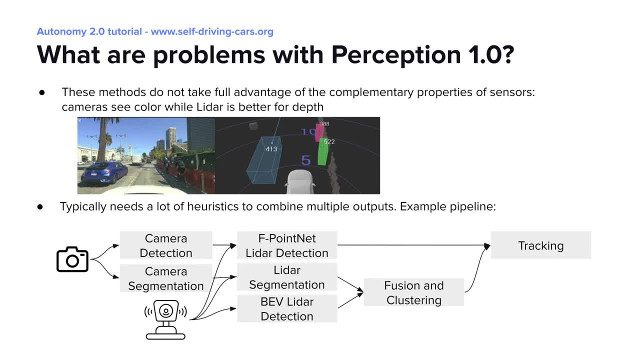 heuristics such as threshold tuning. This makes scaling and optimizing stack very challenging. The bottom diagram shows an example real perception stack that fuses many LiDAR and camera models together. You can imagine the complexity of the code and infrastructure required to tune. 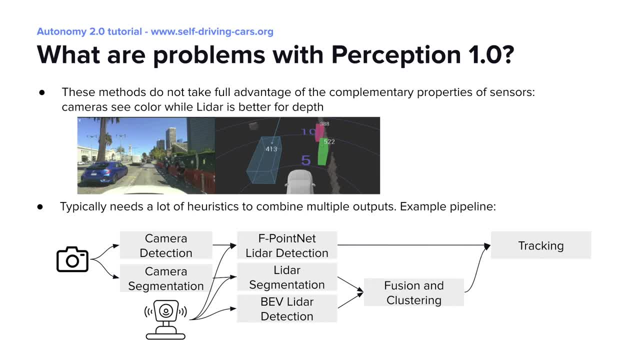 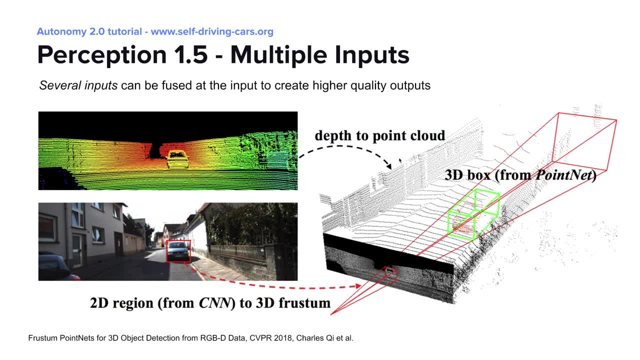 update and deploy this kind of stack in production. Next, keeping these problems in mind, let's move on from single modality models to multi-modal solutions. One of the most famous examples is f-point net. This model uses the outputs of 2D object detection to cover up frustums in the LiDAR space and then produce point. 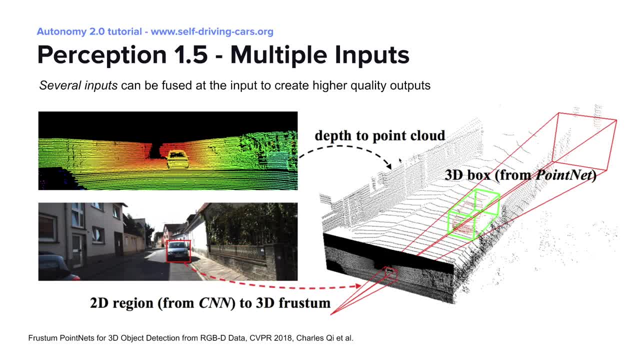 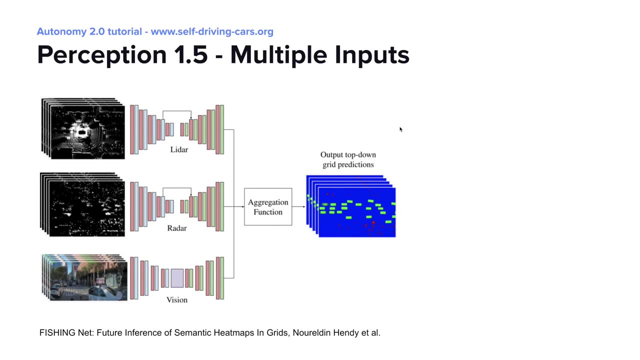 classifications and 3D detections on top of these frustums. This is a very common example of taking advantage of the strengths of detection in RGB color space with the accurate depth of information from LiDAR. Another example of a multi-modal solution is fishing net. This model tries to treat 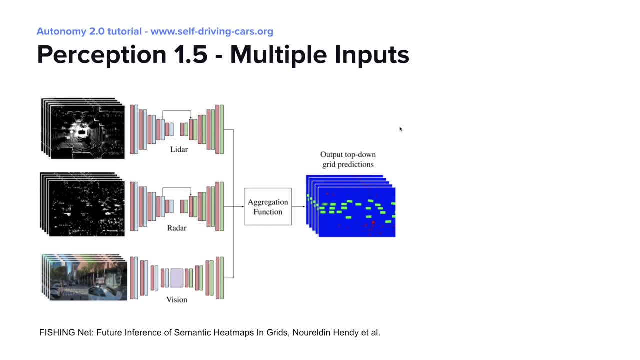 all sensors equally by mapping them to the same space with 2D confidence. The mapped features are then aggregated to produce top-down or bird's-eye view semantic key maps of the scene. The model also aggregates temporal frames for each sensor and then produces a sequence of short-term predictions. 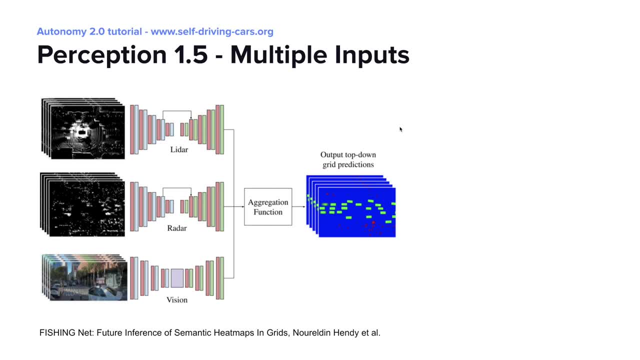 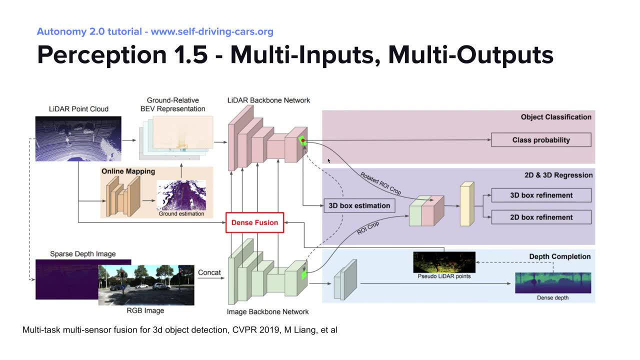 that can then be used for raster-based downstream tasks. As a last example of multi-modal fusion, here we show a network that fused LiDAR and camera inputs to simultaneously output 3D bounding boxes and dense depth maps. This model shows that the same 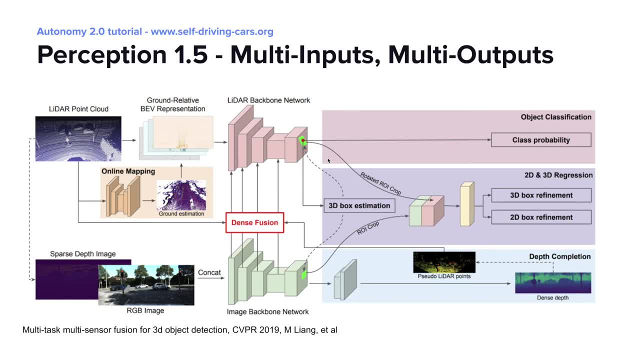 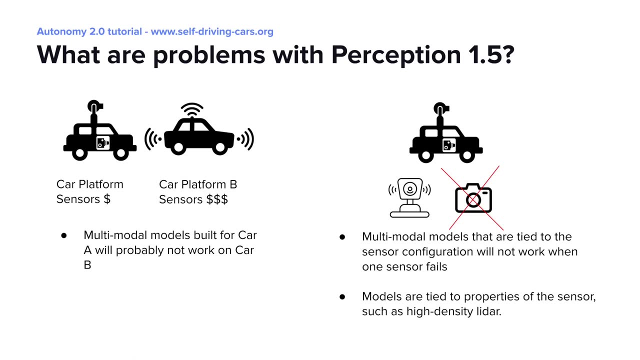 type of complementary advantages of f-point net can be achieved with an early fusion method. In addition, adding auxiliary loss predictions, such as depth completion, can actually help the network generalize. So what are the challenges with these multi-modal methods? One problem is that they're not generic. They typically rely on a fixed set of sensor inputs. 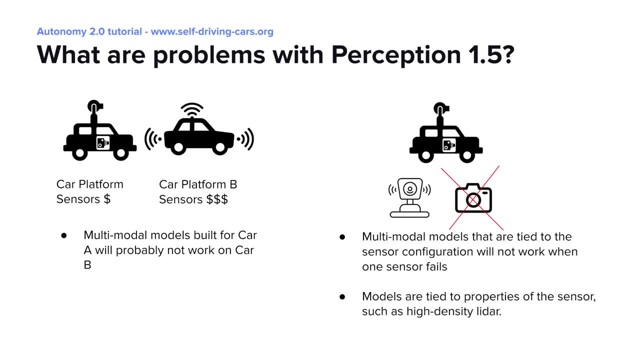 and do not allow scalable development of perception when the sensor is updated, which can be as frequent as when new hardware replaces older ones. As another example, let's say we want to build an Atomy stack for a car running on high-quality sensors. 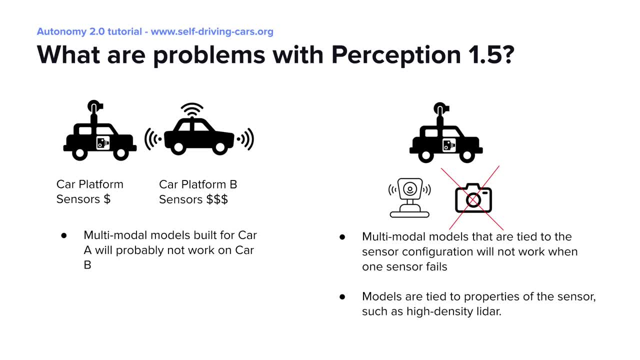 but later we want to lower the cost to run on budget sensors. The same models will not likely work. Additionally, they'll probably stop working if one of the sensor inputs fail. For example, a camera LiDAR model twinned together will typically not work when either. 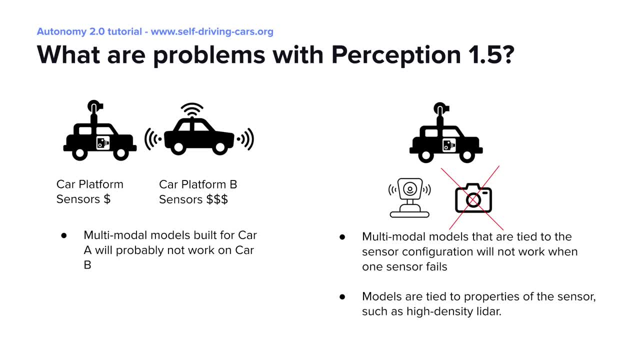 of the sensors is missing. Models are also heavily tied to the physical property of the sensors. For example, the majority of LiDAR models today have an implicit amount of f-point net and have an implicit assumption on a high density LiDAR and the ability to infer. 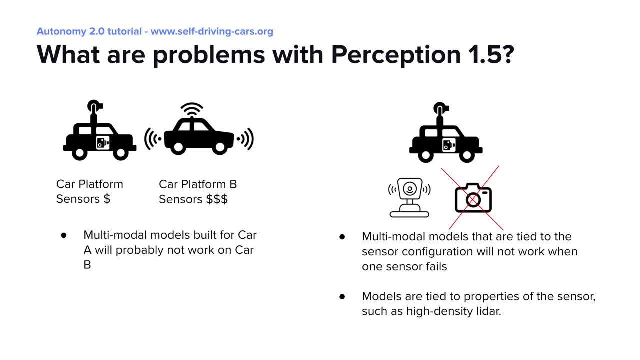 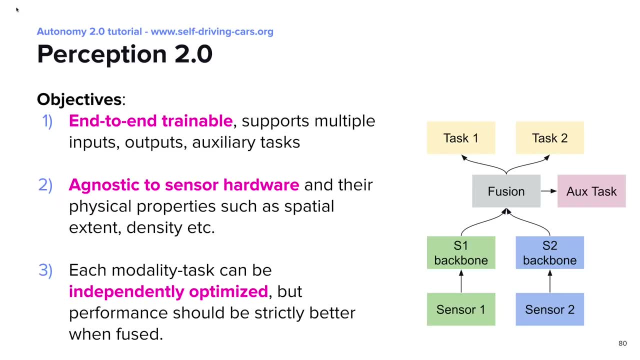 structure from LiDAR alone. What if we want to deploy models on sparse LiDARs? So for the next generation perception system? we can distill down to a few objectives. First, we want the stack to be end-to-end trainable with multiple inputs. 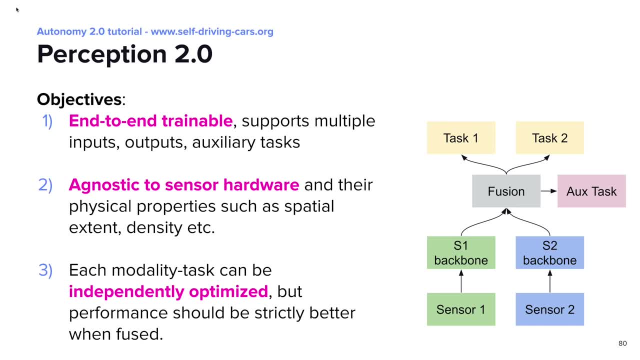 outputs and auxiliary tasks. These outputs should then feed directly into the planner. This will, in turn, allow us to avoid heuristics and glue cold. The stack should then be agnostic to sensor architecture and the physical properties. It should work together whether we have no LiDAR. 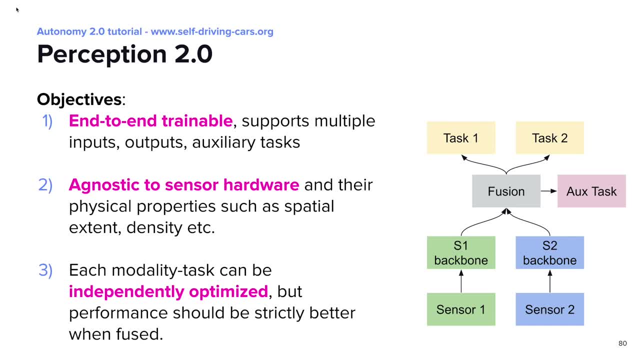 sparse LiDAR or dense LiDAR. This will allow us to scale to multiple platforms. And then, lastly, each sensor or modality should be independently trainable and the performance should increase strictly when fused. This ensures that the stack can. 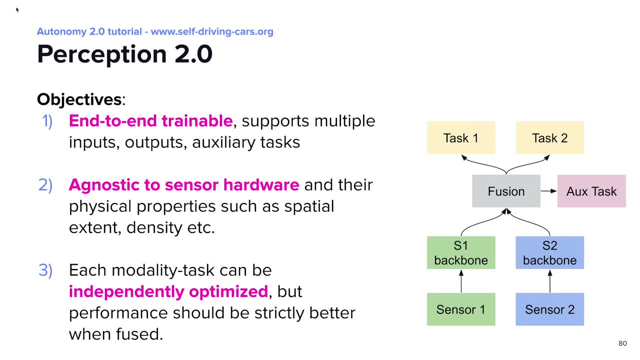 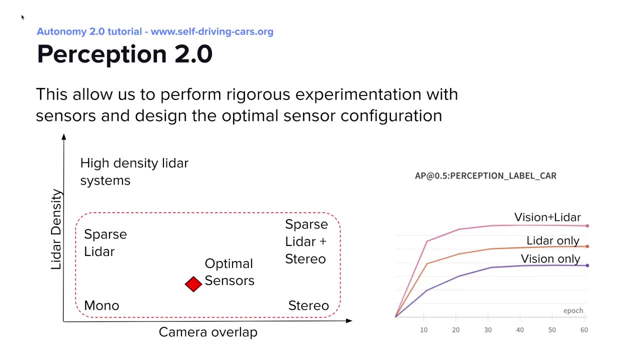 still function when one or more sensors fail. We're calling this type of perception system perception 2.0, and building this at Lyft. So why do we need this kind of system? One challenge we face is that, in order to scale autonomy systems to a large fleet of vehicles, we'll need to build them with cheap sensors. 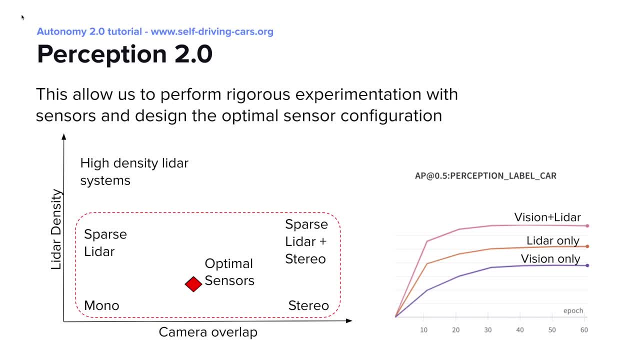 We need to experiment with which sensor configuration really gives us the best performance, perhaps one with sparse LiDAR or monovision or stereo cameras or something in between, As an example, we perform these type of experiments by sweeping across different sensor modalities and trying to 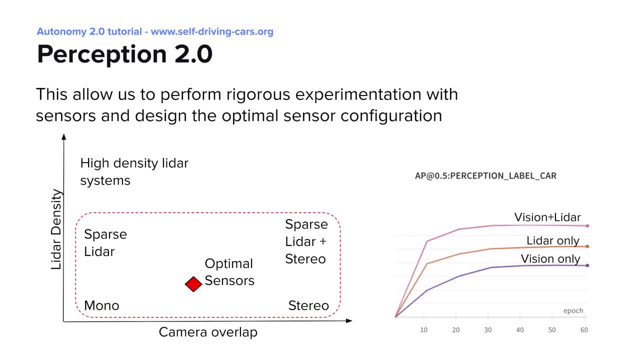 find an optimal set. This is shown in the diagram on the left. The plot on the right shows an experiment where we did this. We build first the modeling model by building a vision-only model, then a LiDAR-only model and then finally fuse them together. We show that overall performance. 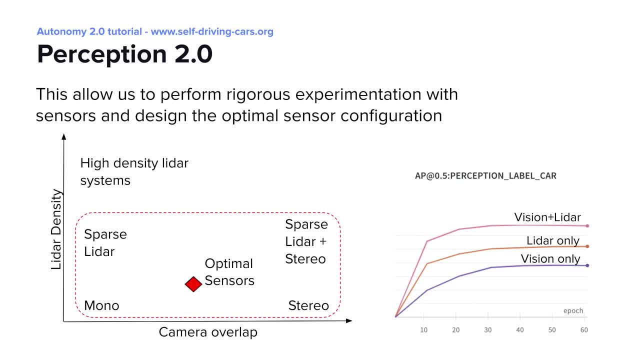 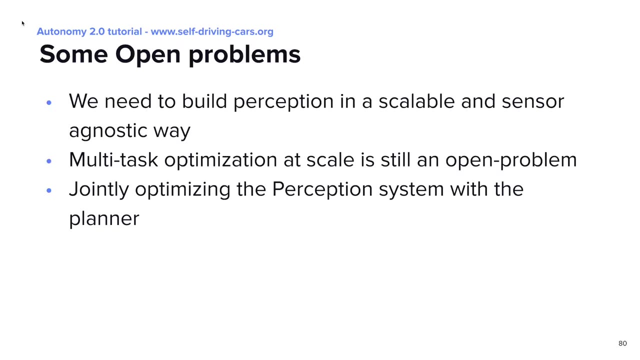 is greater than either of these modes individually. These are all early stage experiments and there are many open challenges in building this type of system. It really presents an exciting opportunity, opportunity for ML and perception. With all the recent advances in machine learning, we've really come a long way since the early days. 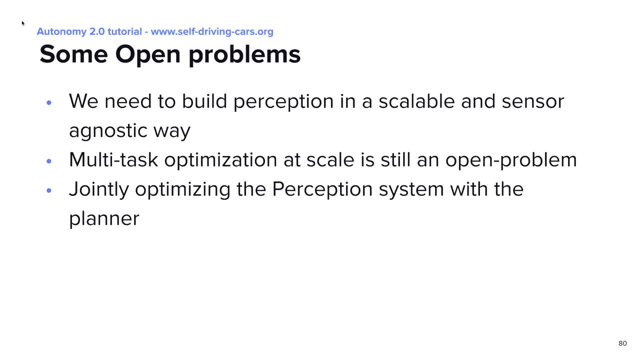 of handcrafted perception systems. However, there are still many challenges that we only briefly touched on or didn't discuss today. First, many self-driving cars demonstrate a high quality perception today, but they're really typically using expensive sensors that will be hard to mass produce. 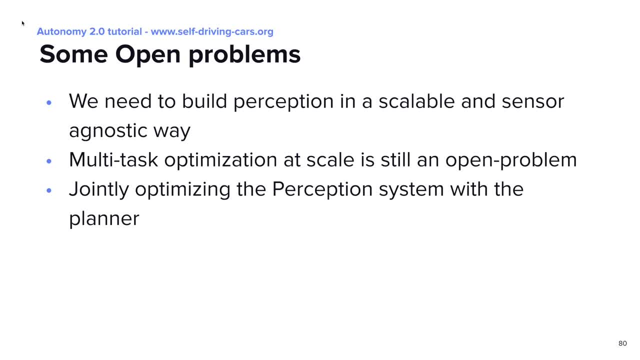 We need our models to be sensor agnostic. We're working on solving this problem at level five, but the challenge very much exists. Second, I want to emphasize that multitask optimization with a large amount of data is very difficult and we need to find solutions that 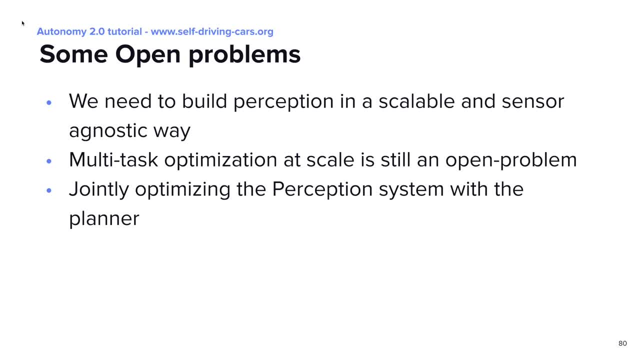 doesn't require manual loss or data balancing. This is an open problem today. Lastly, we typically think of the objective of optimizing perception as perfecting individual tasks, such as localization. However, the true optimization target is really the performance and behavior of the planning. 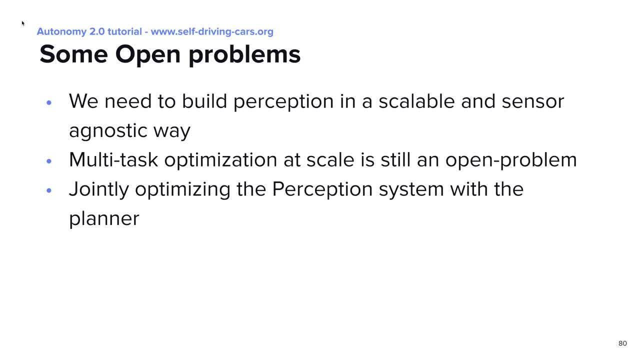 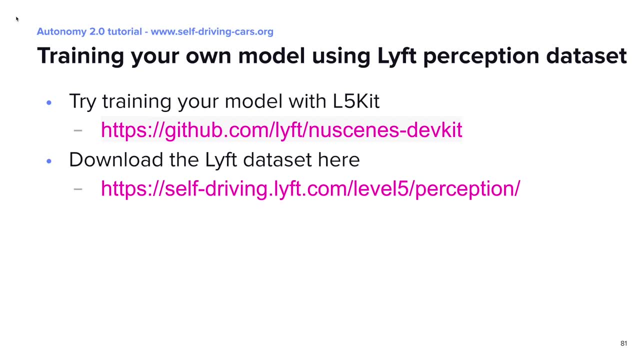 system. These two objectives often don't overlap and we need to figure out how to build perception and planning together. If you're interested in learning more or want to train your own perception model, please check out our L5 kit to help you get started. 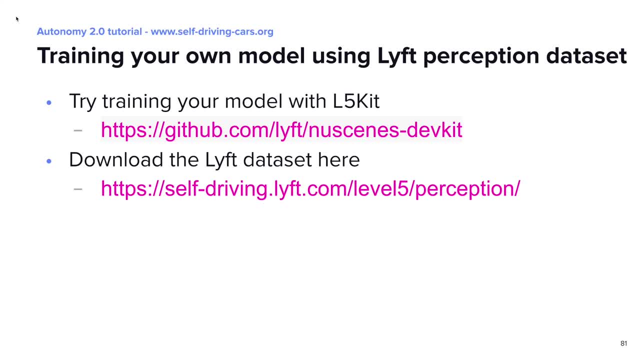 You can also take a look at the lift level five perception data set below.